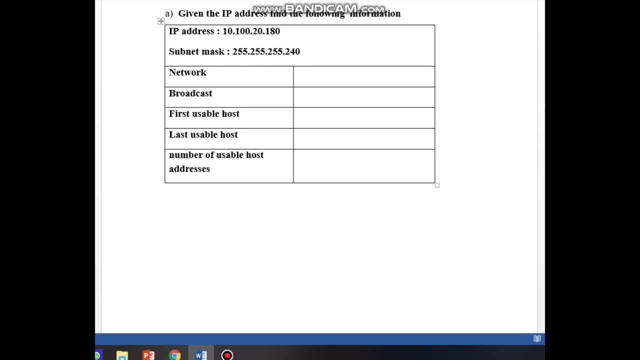 look at the IP address. It has four portions and each portion corresponds to an 8-bit binary number. So 10 will be represented by using an 8-bit binary number. 100, an 8-bit binary number, 20 and 180 will also be represented by 8-bit binary numbers respectively, So 8-bit plus 8-bit. 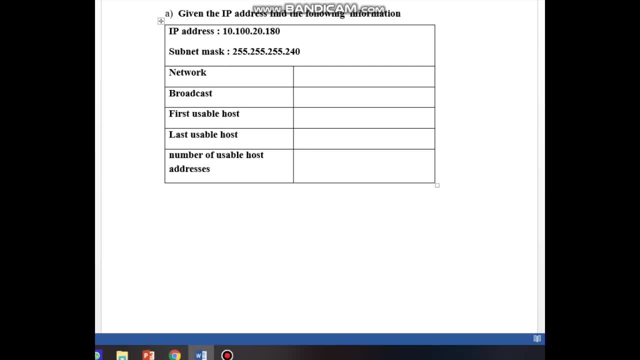 plus 8-bit. plus 8-bit, a total of 32 bits. So 10 bit will be used to represent this IP address, Same for the subnet mask. So let's just first lay that out. So the binary for 10 in 8-bit binary number representation would be 00001010, right. 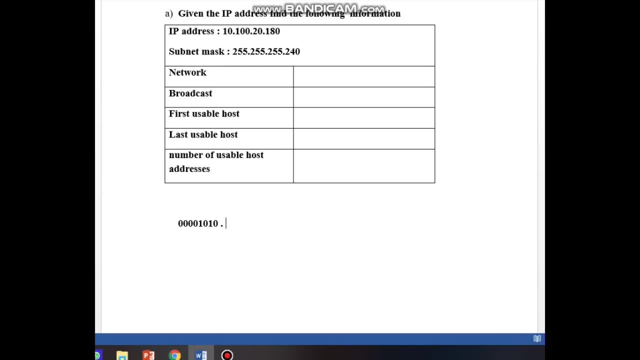 So the binary for 100 will be 01100100.. The binary for 20 will be 0 0 0. 1 0, 1 0 0.. And the binary for 180 will be 1 0 1, 1 0, 1 0 0. 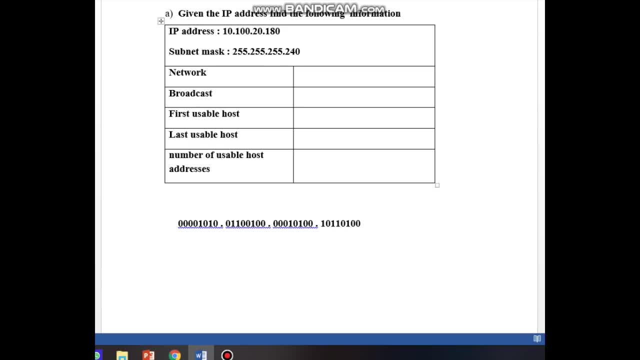 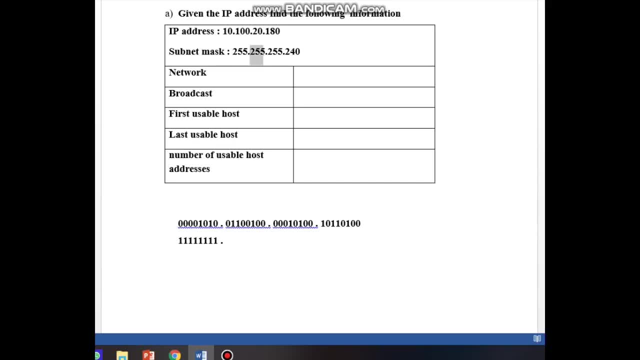 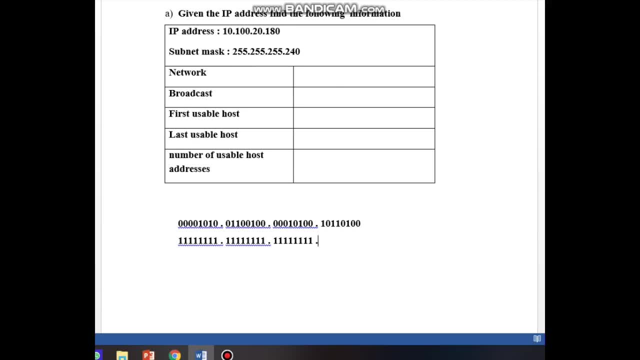 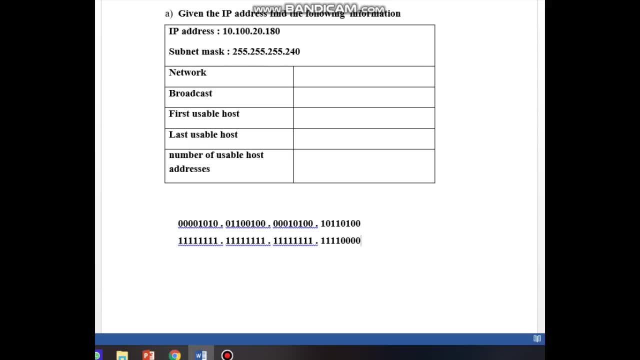 So that's the binary representation of the subnet mask. Now what we have to do is carry on bitwise ending of these binary bits one by one, Right? So let's just go about that. So if we end 0 and 1, so the end operation will only give you a 1 if both the bits are 1.. 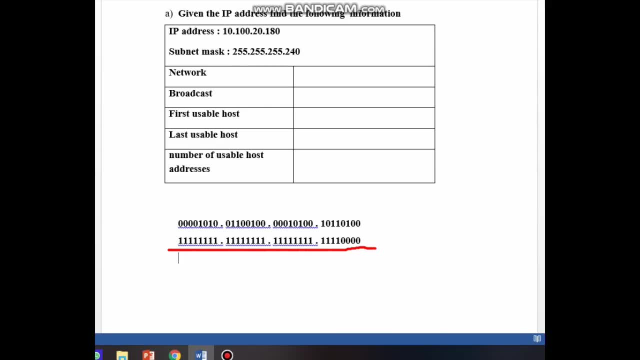 And if any or both of the bits are 0,, then this binary operation, binary ending operation, will give you a 0.. So 0, 1 is 0.. Once again, we have another 0, 1.. So it's 0.. 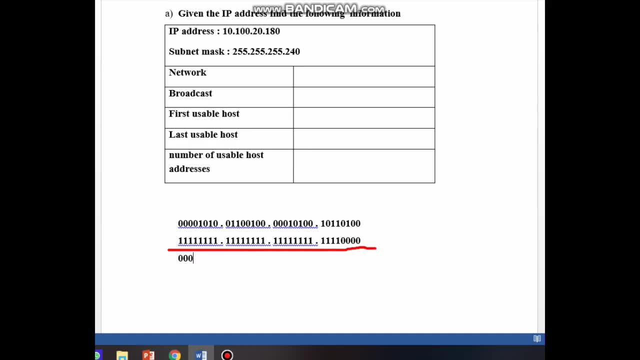 Then we have 0 and 1 here, So 0.. Another 0 and 1.. So 0.. Then we have 1, 1 here. So carrying out the end operation will give you a 1.. We have 0 and 1.. 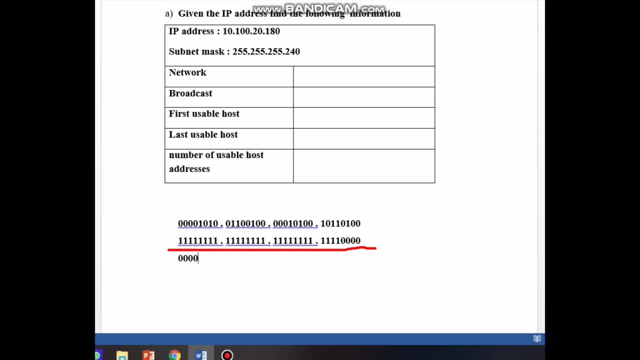 So that's 0.. That's another 1 there and 0.. Right, So if you see over here, let's just inspect this a little bit. So in the first octet we had 0, 0, 0, 0, 1, 0, 1, 0.. 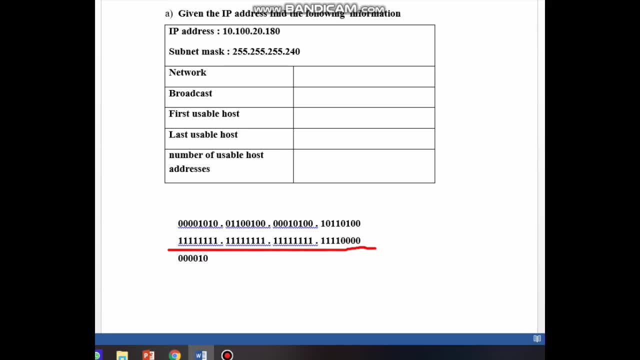 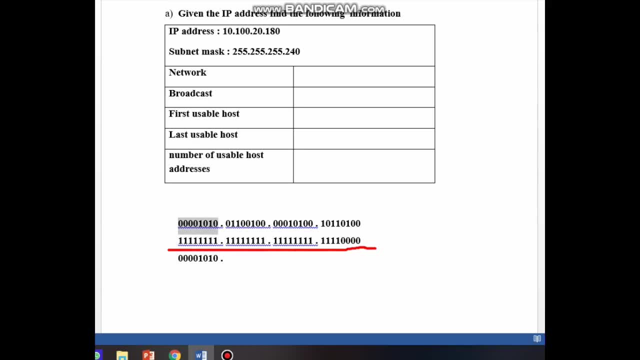 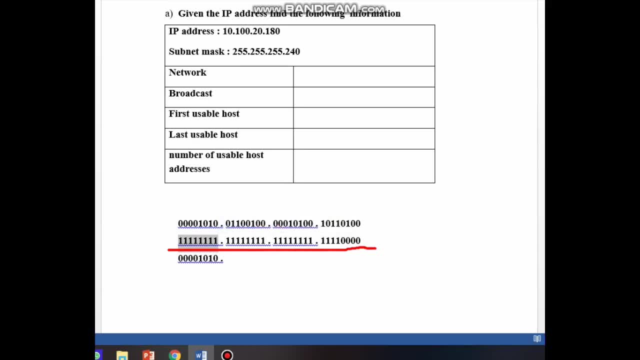 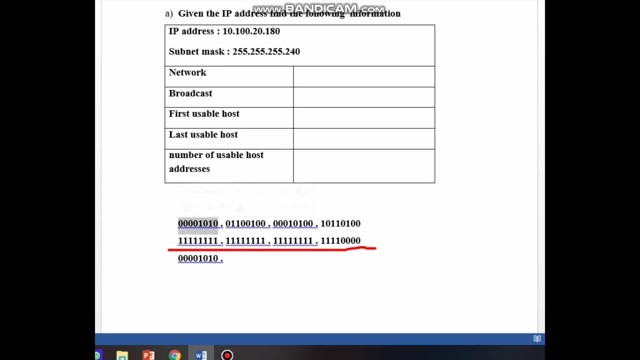 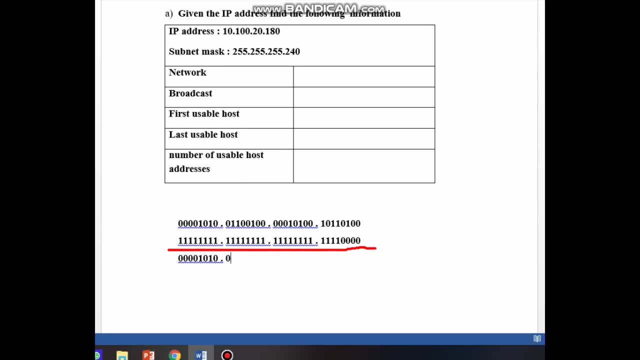 That's what we just had initial. So similarly We do this ending operation in the second octet: 0, 1 0.. 1, 1, 1.. 1, 1, 1.. 0, 1, 0.. 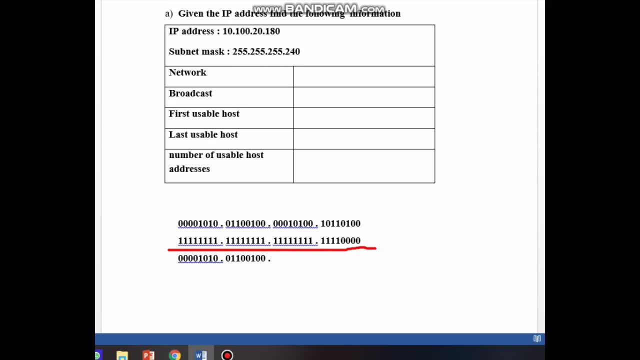 0, 1 0 0.. So once again we ended up getting what we just had initially Right, all ones. so we can pretty much guess what's going to be. just what we initially had: 0, 0, 0, 1, 0, 1, 0, 0 right, but in the fourth octet we do not have all. 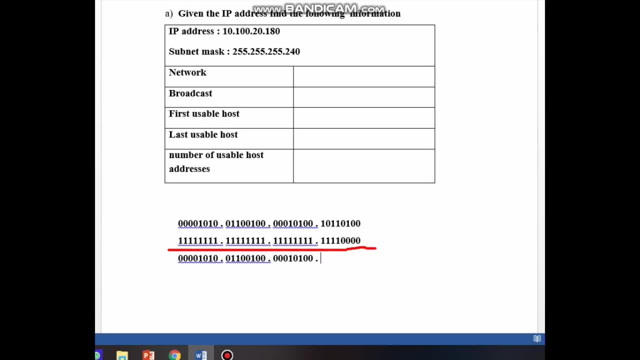 ones, so there might be few changes in our output, right? so we have 1- 1, that's going to be a 1. we have a 0- 1, that's going to be a 0. we have another 1 and 1, so 1. once again 1 and 1, so 1. then the rest of the 4 bits is going to just be. 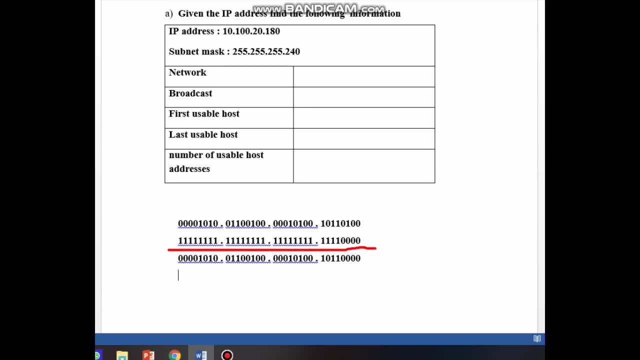 0 right. so now, if we just write the decimal representation of this, we will be getting our network address right. so 0 0 0 0, 1 0, 1 0, that's just 10 0 1, 1 0 0. 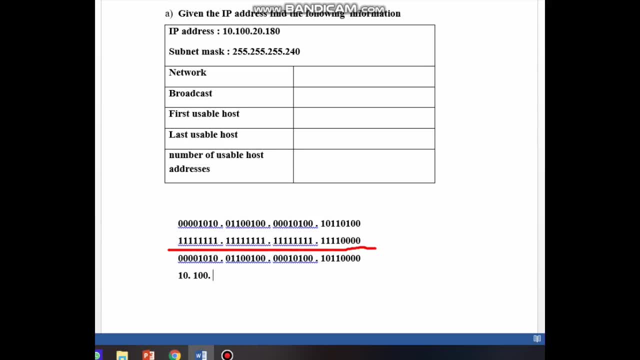 1 0, 0, that's 100, right? this one third octet is just going to be 20. the fourth octet, that's going to be 176, right? so this is going to be our network address. I can just write down here: our network addresses 10, 100, 20 dot. 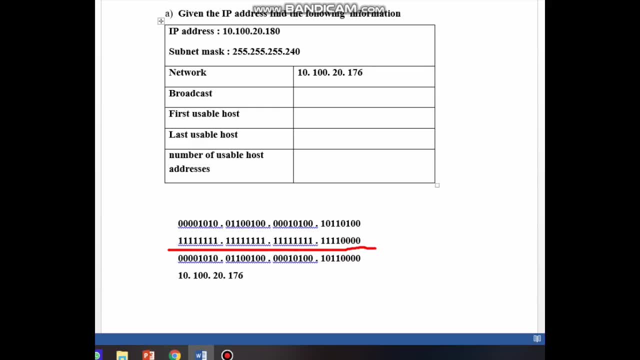 176. right, so another thing to do, guys. let's look at this subnet over here. so in the subnet mask we have all ones in the first octet, all ones in the second octet, all ones in the third octet and only four ones. 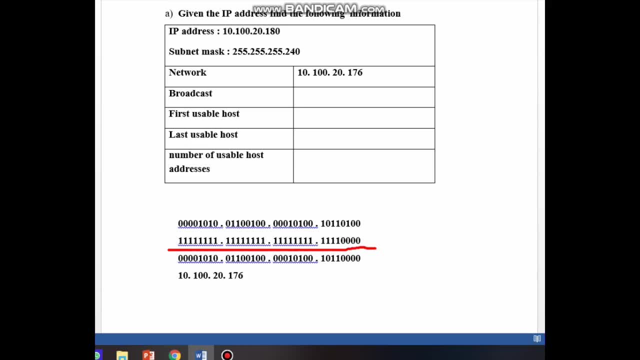 in the fourth octet. So the prefix max for this will be the number of ones that we have, right? So this is 8 plus 8 plus 8 plus 4, so that's going to be 28,, right? So what? this subnet mask. 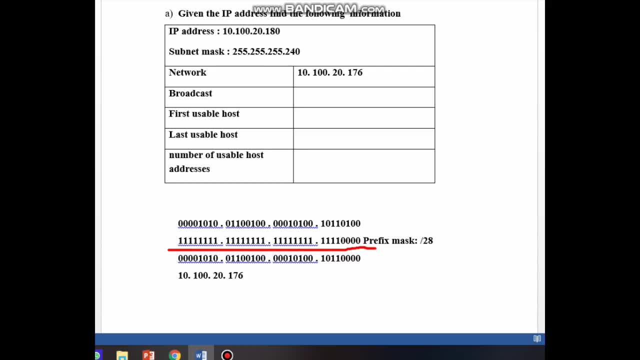 tells you is a total of 28 bits, starting from left to right is going to be in our network portion right, And the last four bits is going to be our host bits. So, once again, the first 28 bits is going to be our network bits and the last four bits is just going to be our host bits. 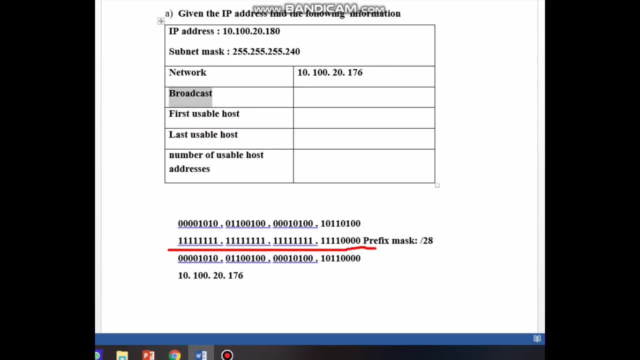 right, So we get the broadcast address when we set all the host bits to one. So right, So these four bits over here, these are our host bits. right, So I will get my broadcast address when I turn all my host bits to ones. 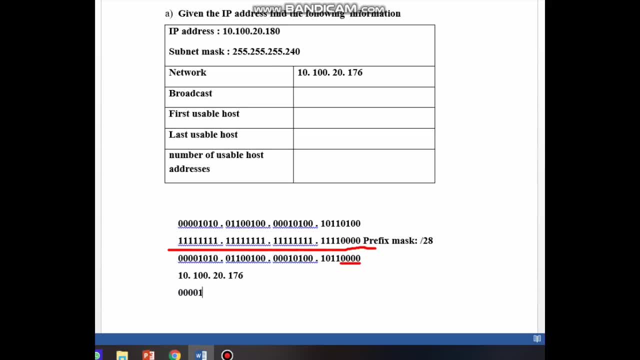 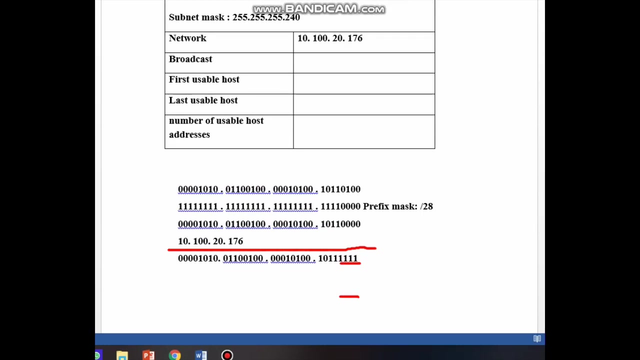 So if I do that, what I'll be getting is 00001010.01100100.0010100.101111111.. I just turned all my host bits to ones right, So now, if I write the decimal representation of this, it will be 10.. Then I'll get my broadcast address when I turn all my host bits to ones. So now, if I write the decimal representation of this, it will be 10.. So now, if I write the decimal representation of this, it will be 10.. 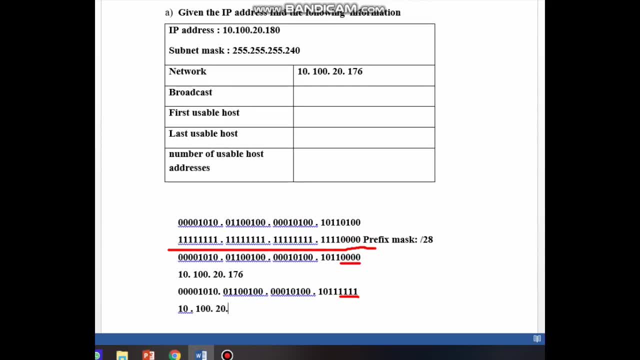 So now, if I write the decimal representation of this, it will be 10.. 100.20.191.. Just doing the decimal representation of this, right. So I'm just going to write my broadcast address. It's going to be 10.100.20.191, right. 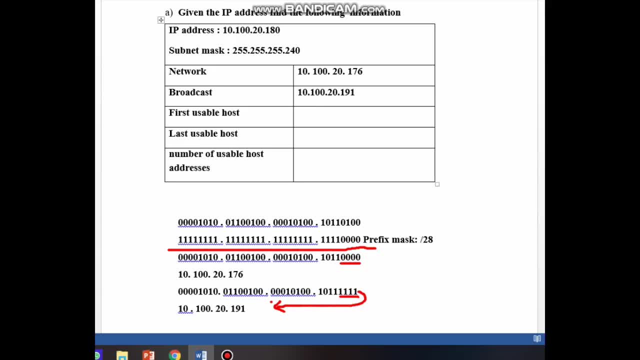 So my first user host is the address that's immediately after my network address, right? so in other words, it will be when I turn this very last host bit to one. so if I write it like one zero one, one, zero, zero, zero one, that's going to be my very first. 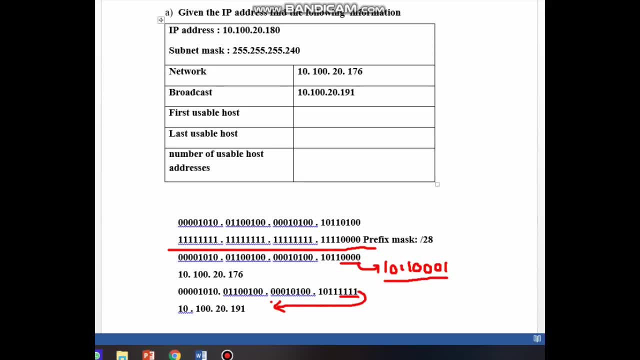 host address. the rest of the portion stays the same. so my very first usable host is just going to be the address immediately after. my network address is going to be 10.100.20.177, so my last usable host is going to be that one. 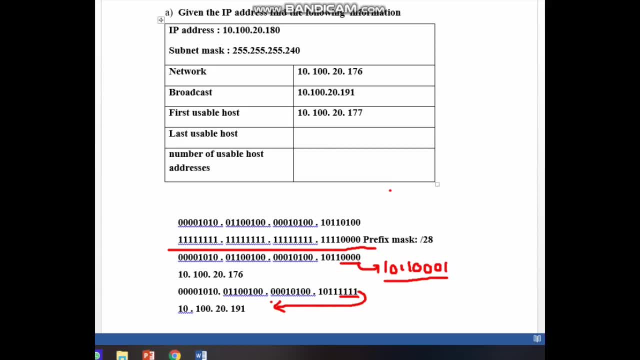 host. it's immediately before my broadcast address and if you look into our broadcast address, the address that's going to be immediately before my broadcast address is just going to have a zero in this very last bit. so it's just going to be one zero one, one, one, one, zero, one. sorry, one zero, right? so if 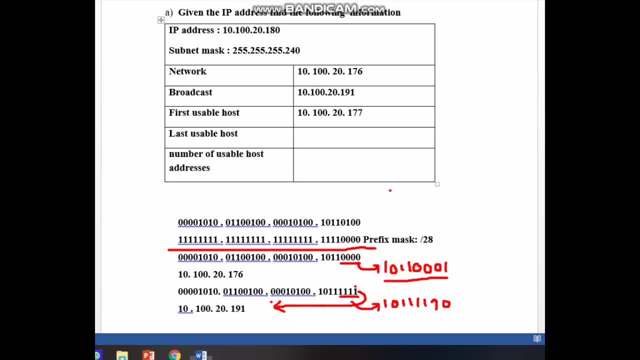 we just write the decimal representation of this, that will be 190. that's the address that's immediately before my broadcast address. right, so it's just going to be ten dot, hundred dot 20.. O, 190, right. So if we're done with that, what we can look into now is: how many hosts can we? 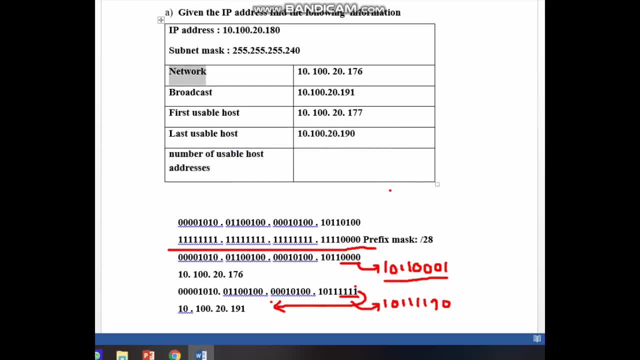 accommodate using this network address, right? So, if you think about it, the network address and broadcast address, right. We cannot assign this to any particular devices, right? But everything that's between the network address and the broadcast address we can give to any host. 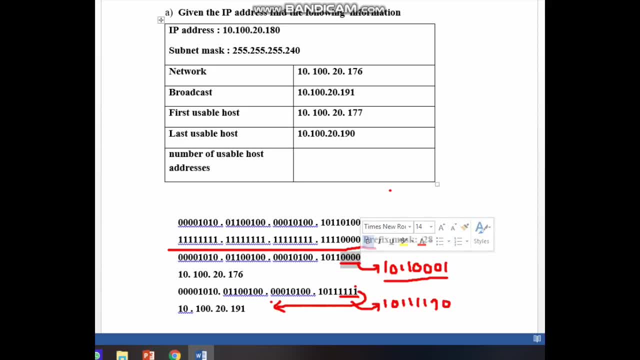 So the host bits we had over here we had four host bits and these host bits can be written. since we have four host bits, So it can have a combination of two to the power four, right, So that's 16 combinations. But when the host bits are all zero, that's just going to give you the network. 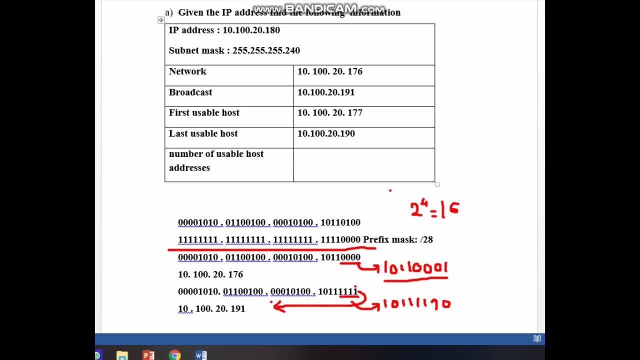 address And when the host bits are all ones, it's just going to give the broadcast address. So two of these addresses we cannot use. So the number of usable hosts will be 16 minus two, which is just 14, right? So the number of usable hosts will be 14.. So that's about it, guys. I hope it helped you. 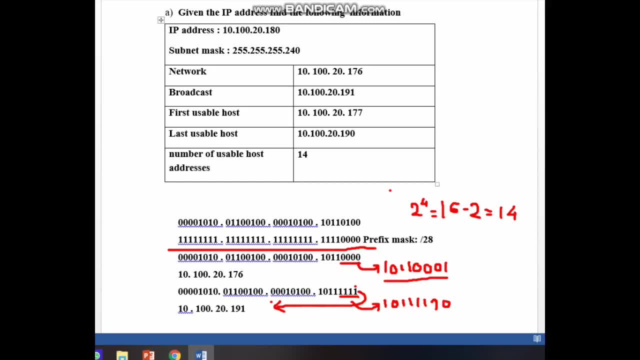 understand The problem a bit And thank you for watching.